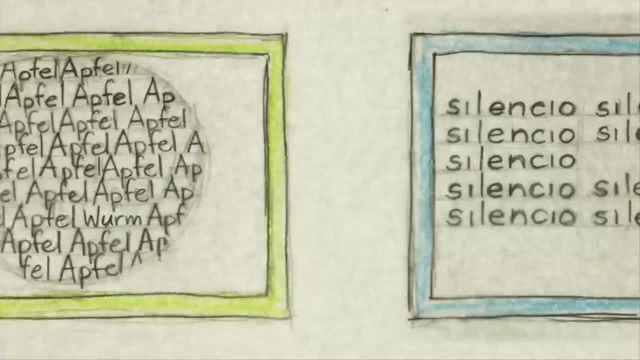 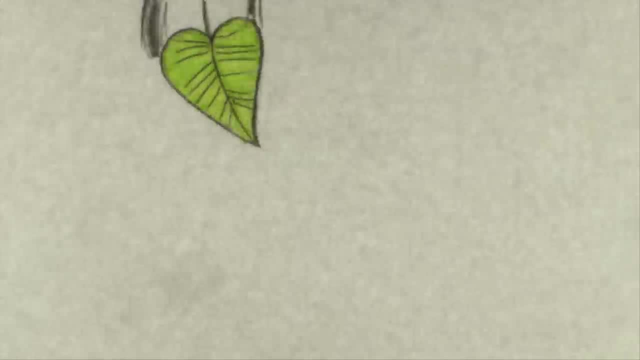 a poem doesn't need to be lyrical. Reiner Doell's Abfell and Eugen Gommringer's Silencio toe the line between visual art and poetry. Meanwhile, EE Cummings wrote poems whose shapes were as important as the words themselves. 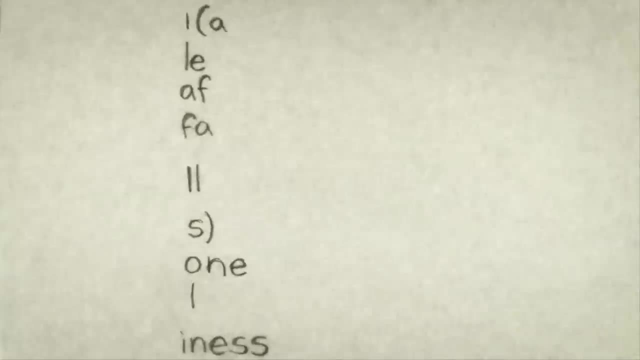 in this case, amplifying the sad loneliness of a single word, a single leaf falling through space. If the visual nature of poetry faded into the background, perhaps we'd be left with music, And that's an area that people love to debate. 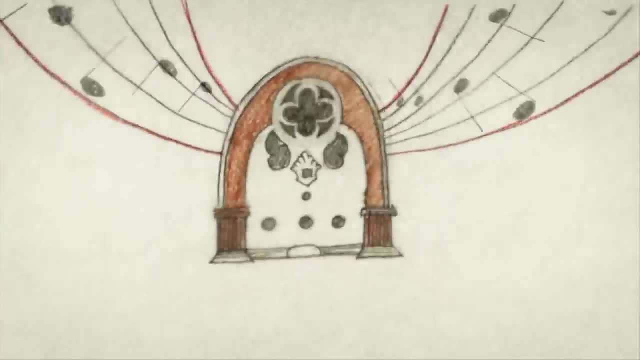 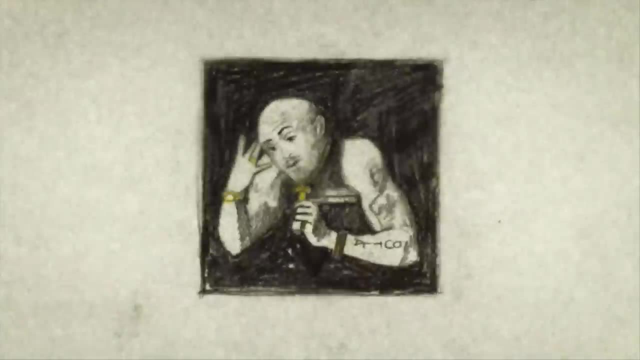 Are songs, poems. Many don't regard songwriters as poets in a literary sense, but lyrics from artists like Paul Simon, Bob Dylan and Tupac Shakur often hold up even without the music. In rap, poetic elements like rhyme, rhythm and imagery. 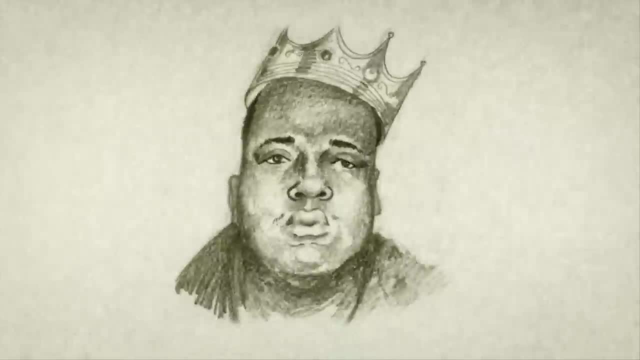 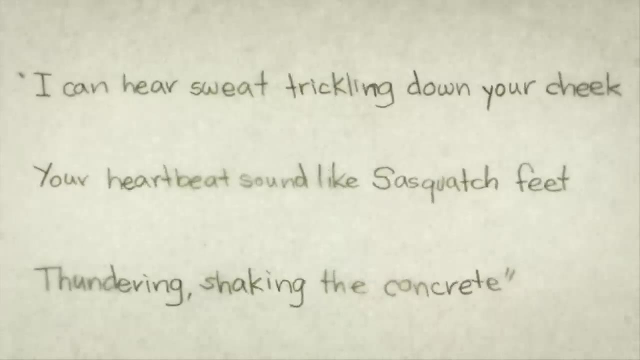 are inseparable from the form. Take this lyric from the notorious BIG. I can hear sweat trickling down your cheek. Your heartbeats sound like Sasquatch feet thundering, shaking the concrete. So far, all the examples we've seen have had line breaks. 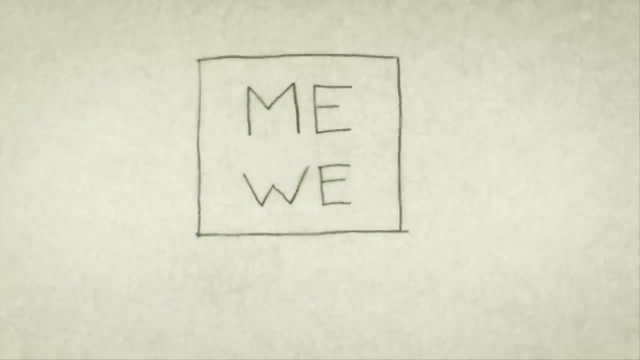 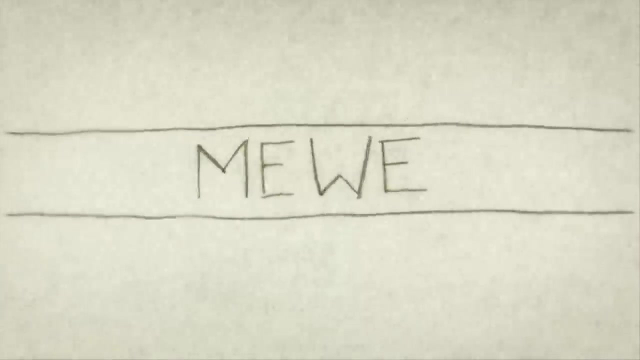 We can even imagine the two words of Ali's poem organizing in the air me we. Poetry has a shape that we can usually recognize. Its line breaks help readers navigate the rhythms of a poem. But what if those line breaks disappeared? Would it lose its essence as a poem? 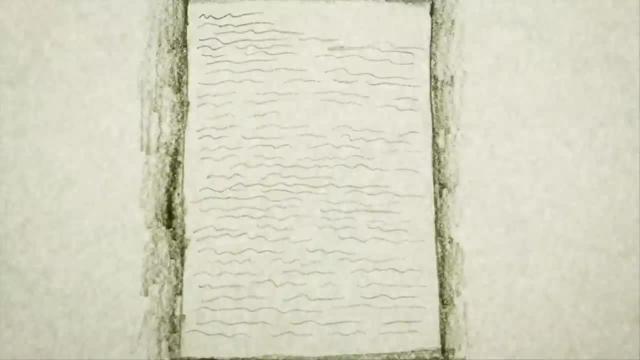 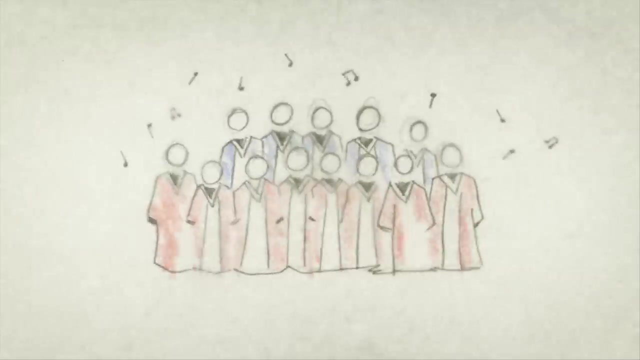 Maybe not Enter the prose poem. Prose poems use vivid images and wordplay, but are formatted like paragraphs. When we look at poetry less as a form and more as a concept, we can see the poetic all around us: Spiritual hymns, the speeches of orators like Martin Luther King Jr. 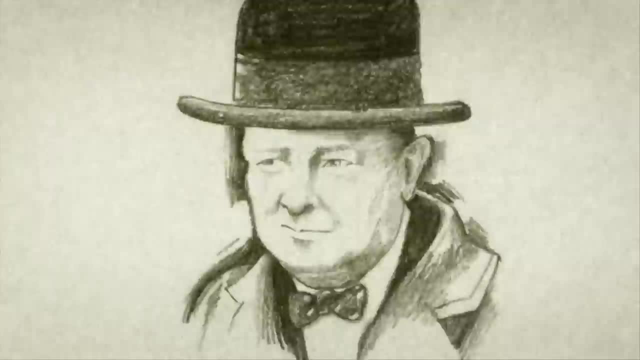 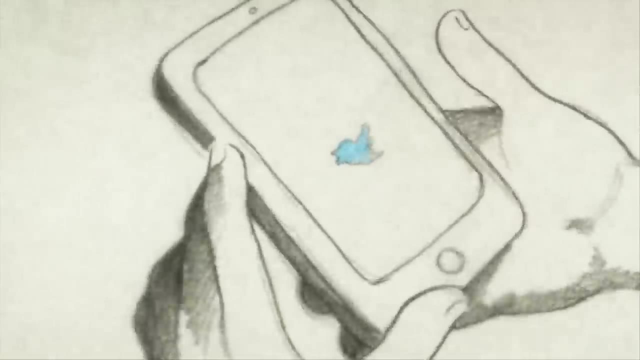 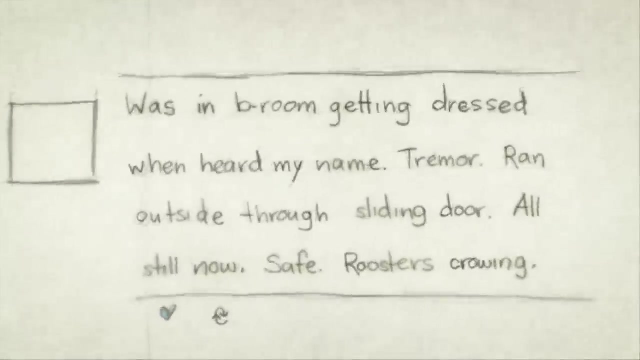 JFK and Winston Churchill and surprising places like social media. In 2010,, journalist Joanna Smith tweeted updates from the earthquake in Haiti. Was in B-room getting dressed when heard my name, Tremor, Ran outside through sliding door. All still now. 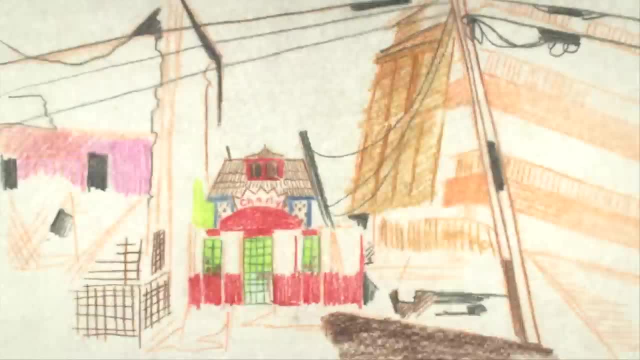 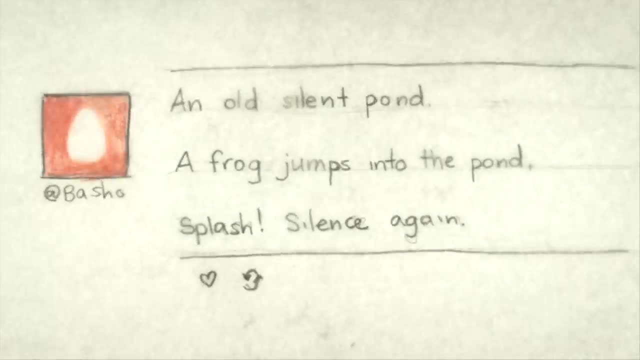 Safe Roosters. crowing Smith uses language in a way that is powerful, direct and filled with vivid images. Compare her language to a haiku, the ancient Japanese poetic form that emphasizes bursts of brief intensity, with just three lines of.